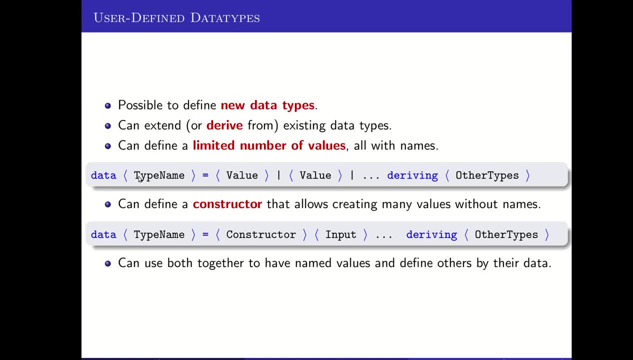 countries in our type name, and our type name might be country, For instance, and then we can state what other existing types they are deriving from, and we'll see some examples of that. And then another way that we can define our data types is to define: 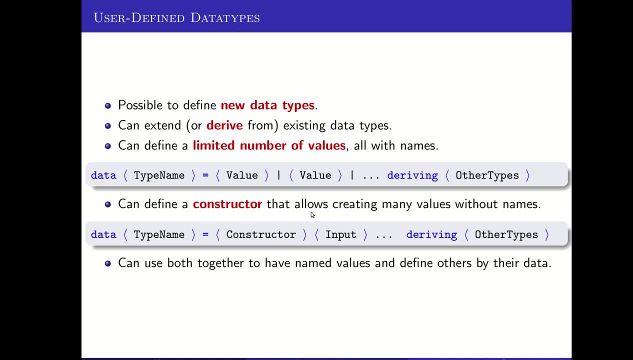 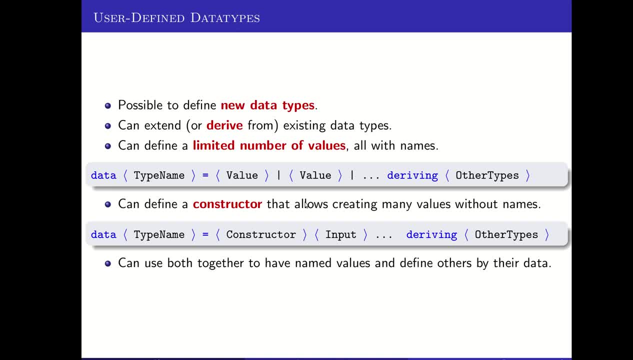 we may store them as variables with names, but they don't automatically get names. like you know, China or United States or things like that- The values would have in our first example. We can, however, mix and match these two If, for instance, we had some predefined named ones. 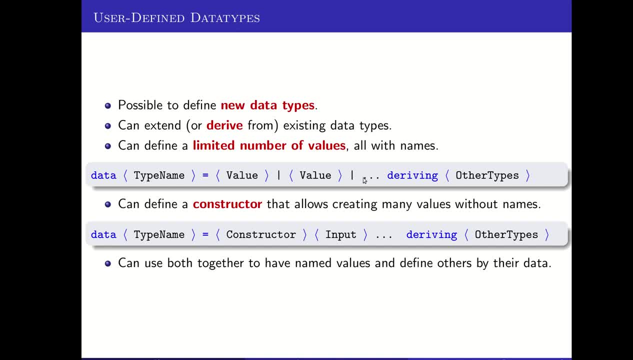 that we knew we wanted to make sure got included. we could include those And then we could just put a bar and some constructor types that would allow us to build, you know, a larger number, probably unlimited number, of possible types, using ints or strings or whatever as the inputs to those, And we'll see examples that are. 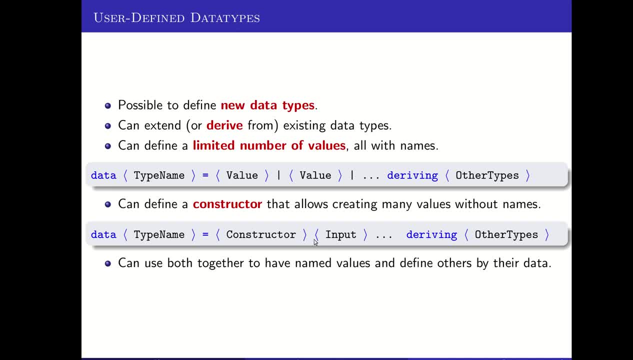 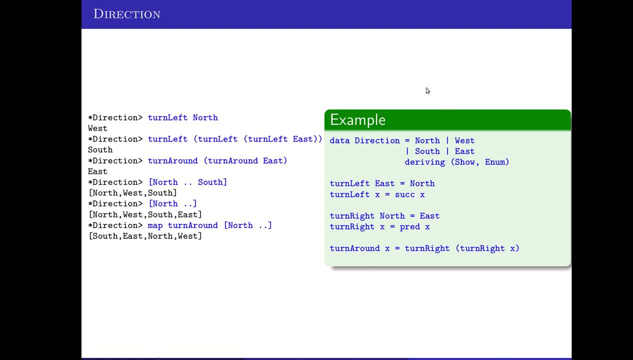 purely one of these or purely the other, and some examples that do mix and match the two of them. So here's one example that uses only named types. It's the direction type that I've defined here that has only north, west, south and east. The ordering of these mattered in the example I'm. 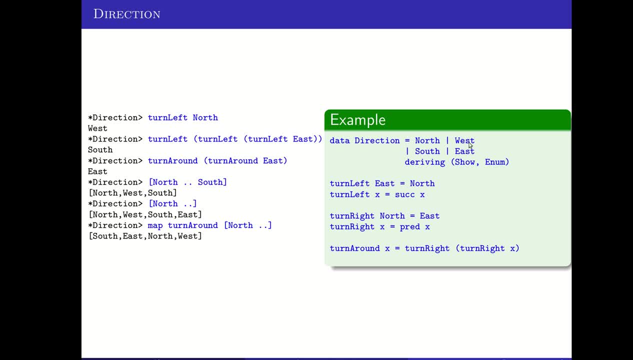 doing here. It won't always matter what the ordering is, but in this case the ordering does matter because I've derived from the enum type. That's a type that allows us to enumerate between the values, like how we can enumerate between integers or things like that. I've also 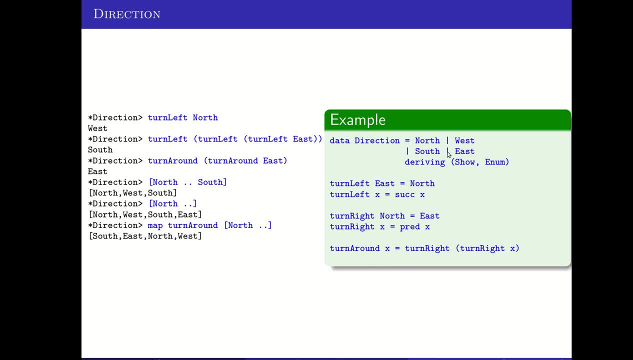 derived from the show type, which will automatically allow them to be shown according to the names that were given here or according to how they were constructed. if we use the constructor types, which this one doesn't have, I've then defined a few functions for them, So you can see that. 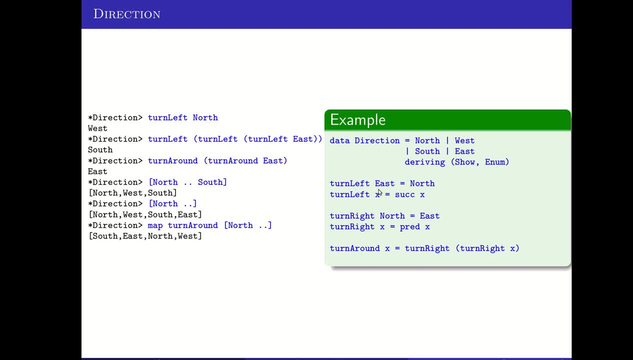 turn left of most values, can just ask for the successor of that value. So for north, the successor would be west. For east, however, there is not a successor. An enum does not loop back, just like the integers don't loop back to one. typically They keep going and in this case these aren't infinite, They're a. 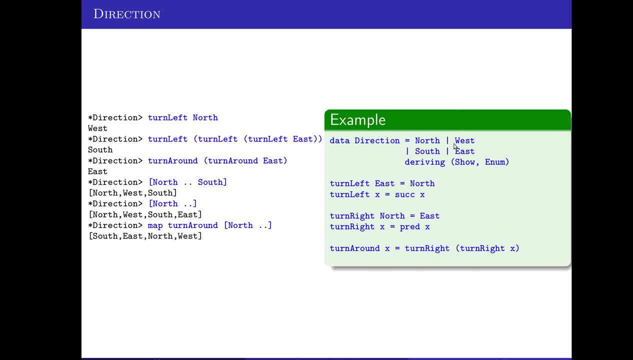 finite set, so they have a limited last value. So if I want people to be able to turn while they're facing east and I want them to be able to turn left, then I need to manually write a case for east and we can do this. 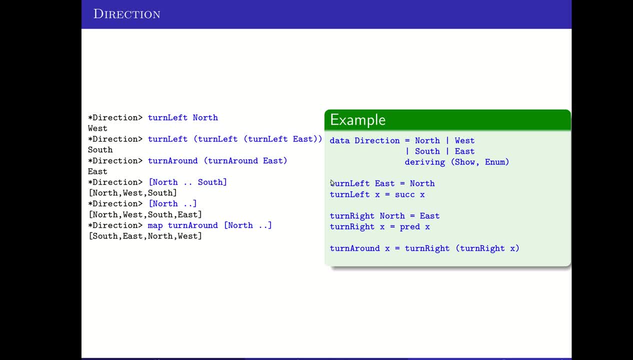 So I'm going to write a case for east on our type names there, and Haskell will infer that the turn left function is referring to a direction because of the fact that I'm using east and north in it there. So turn left on north will give me west. If I turn left, turn left, turn left on east, well, we know that the first turn left will give me north, then west, then south, and so south will be my result. 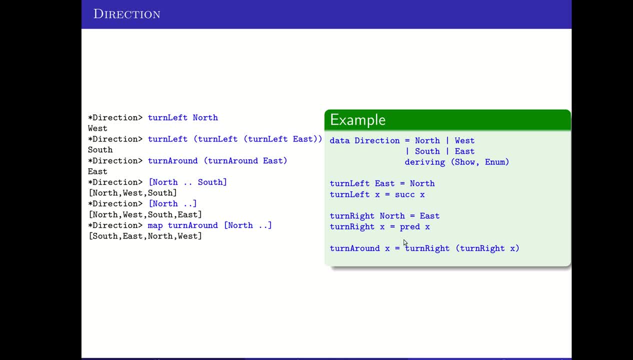 You see, I've defined turn around as turning right twice and that turning right needs a special case to go from north back to east. So these are just a few relatively simple functions that I can use for these directions. You can see that because I derived from show, it will show me the types If I don't derive show. 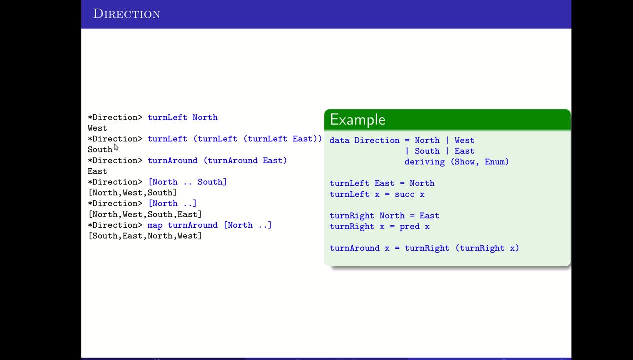 and I try to display a result, then it's going to: I'm going to get errors, that there's no way to show those results, that type. Another interesting thing that I can do, because this is an enum type, is I can do those. 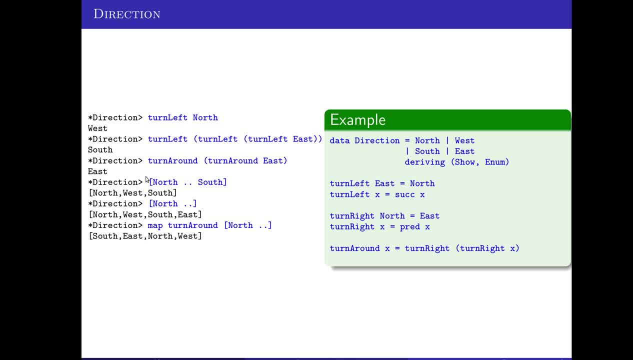 ranged lists, where I create a list from north to south and it will go northwest south. I can create a list from north to unlimited, but it will be limited because enums are typically limited. If I wanted one that went further, then I might have to do some tricks with my turn, left or turn. 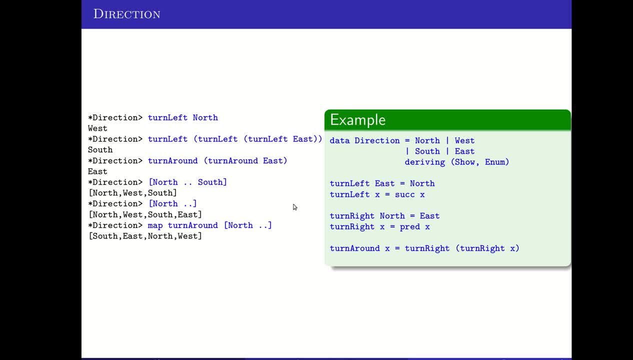 right to be able to get more than just those. If I wanted to take eight turns, then maybe I could map that turn left eight times, or something like that. I can map onto lists of that type as well. So I map, turn around onto it and you see that I get the opposite of each of the directions that 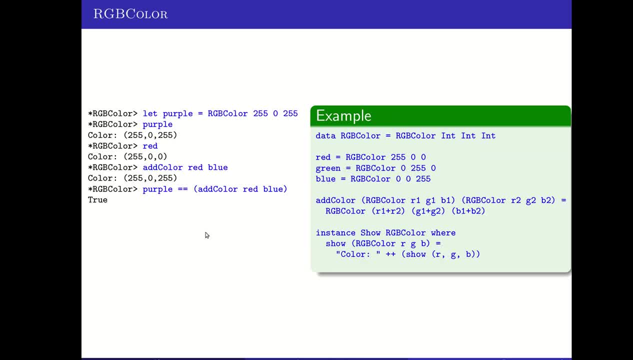 was given there. Here is a data type called RGB color. that is a constructed type. It has no named versions. when the type is declared, It just declares that an RGB color can be constructed from three ints: a red, a green and a blue. 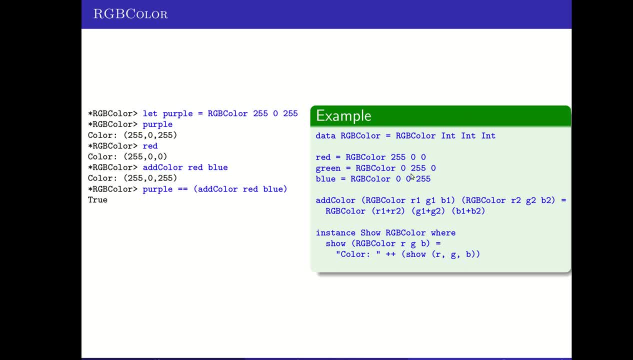 value presumably, And then down below that. I have manually defined a few types. A pure red is RGB color of 255.0.. Then I've defined a pure green and a pure blue. I've defined some functions that work with the RGB color type. So here's add color. It takes an RGB color and it pulls out the red, green and 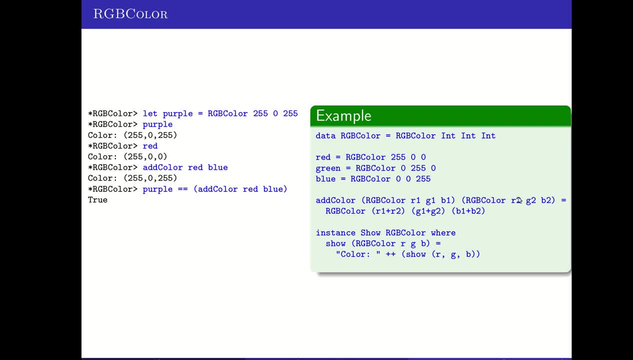 blue from it and then another RGB color pulls out its red, green and blue and then it adds the reds, adds the greens and adds the blues. You'll notice I've done nothing to guard, To make sure, sure that these don't go above 255.. That would be added functionality that I might want to put. 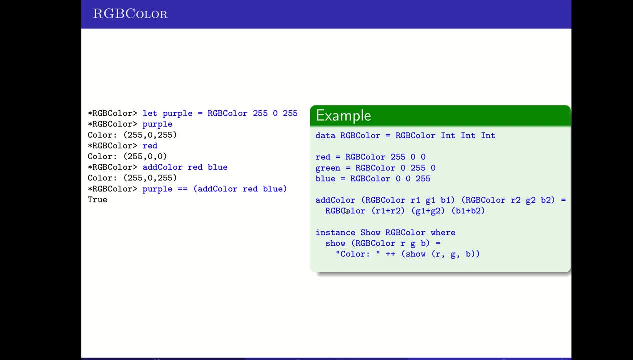 onto this as well, but I didn't do it here. So here I've added: well, here I've manually defined purple to have full red and full blue. but I can also define purple by adding the colors red and blue And you can see that purple is equivalent to the add color red and blue. Okay, And then 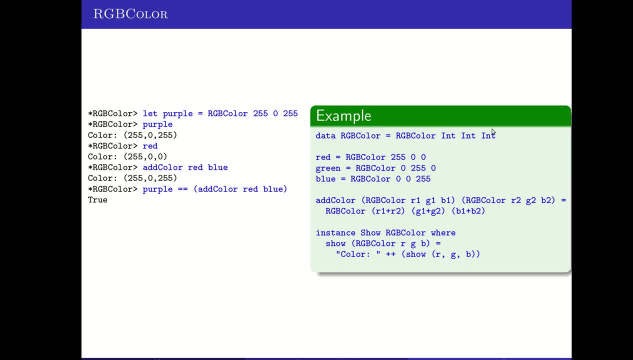 I did not, in this case, derive from show, And the reason I didn't derive from show is because I wanted to manually define how these would be shown. If I didn't manually define how they would be shown, it would simply say RGB color. 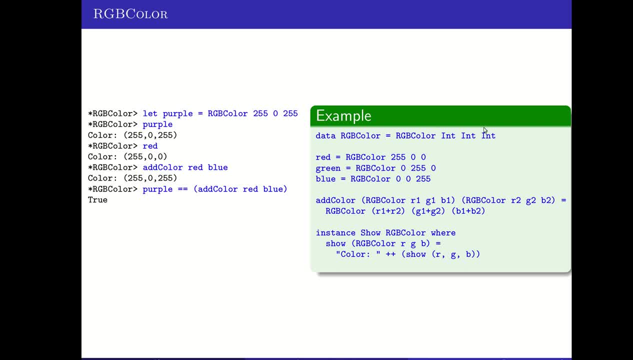 color and then the three numbers. no parentheses or anything, just one statement. So RGB color- 25500, for instance, And I wanted to show a little bit more about it. I wanted to put it in parentheses and some commas and I wanted to have just color. I don't want my users to have to worry. 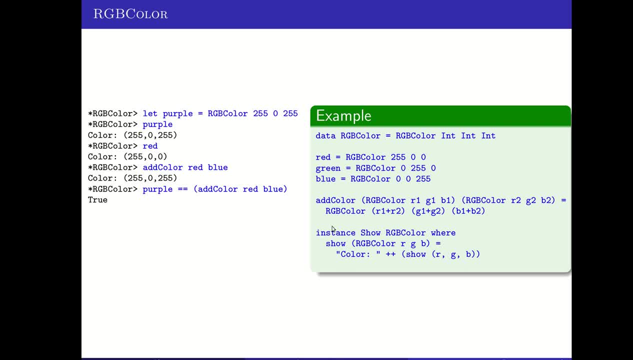 about that. it's an RGB color type, So what I do is, instead of deriving showing, getting that automatic behavior is. I create an instance of show RGB color where the show function for an RGB color breaks out the R, G and B values. It puts on the word color a colon and a space and attaches 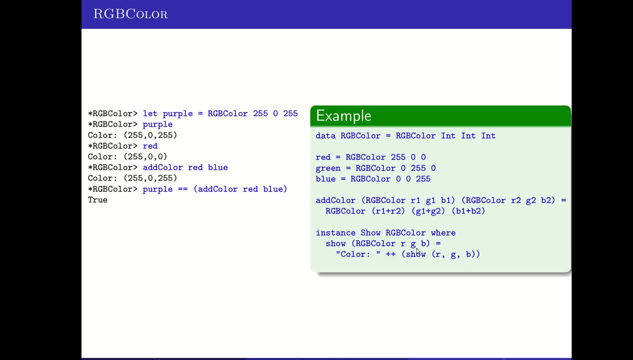 that to the string representation of the tuple RGB, And so that gives us results like the ones that are shown here. And I could do more things like this. I could do more things like this To kind of refine how it was shown in some particular way. 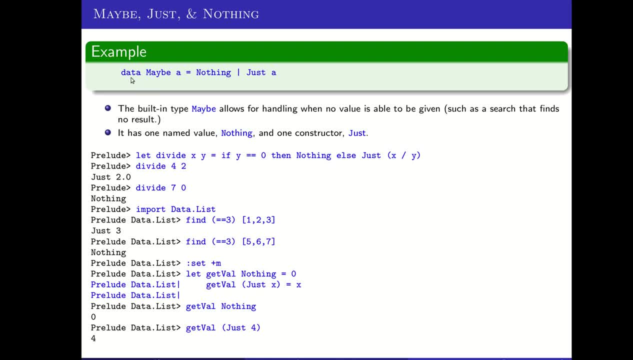 There is a built-in type that gives us some good illustration of type features as well. I'll give you an example of how it could be defined, and this is probably roughly how it's defined in Haskell. But it is a built-in type. You don't have to define the maybe type. In fact. 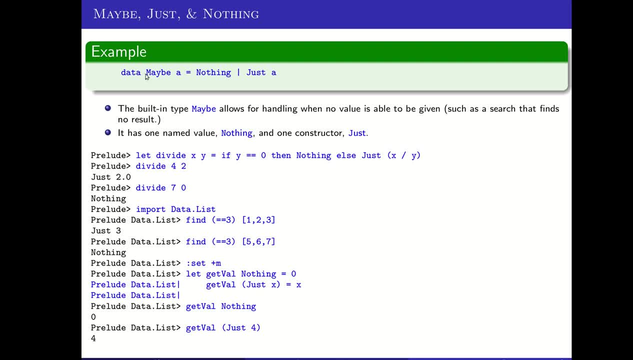 some functions that are built-in type are built-in type So you don't have to define the maybe type. Some functions that are built-in in Haskell already return maybe types, like the datalists find function because it may not find the thing. So the built-in maybe type allows for handling. 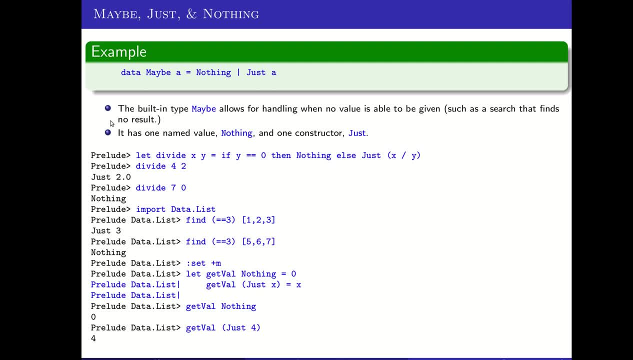 when no value is able to be given, such as a search that doesn't find a result. It has one named value called nothing and then one constructor called just, And you'll see that maybe needs a type that it's going to be storing one of the values that it's going to be storing, And so 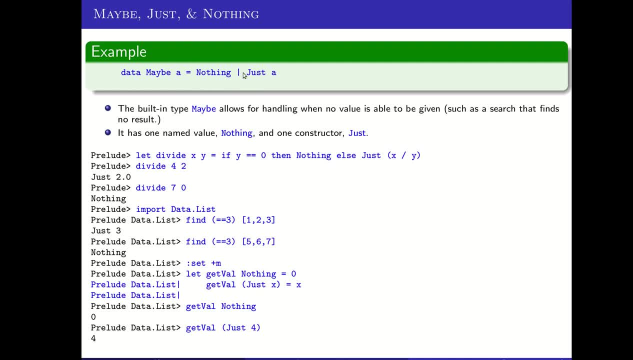 when there is a result. when there is no result, it's just nothing, But then when there is a result, we have a just that has some value. This makes the language a little difficult around this, but it allows us to do things like if we really didn't have a reasonable result to return. 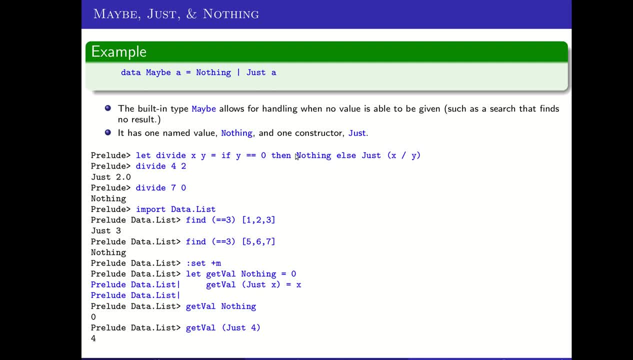 say, returning a negative one wouldn't make sense and returning, you know, an actual number wouldn't make sense. Well, we can return nothing. We can return a divide function that takes an X and a Y. If Y is zero, well, I don't want to just. 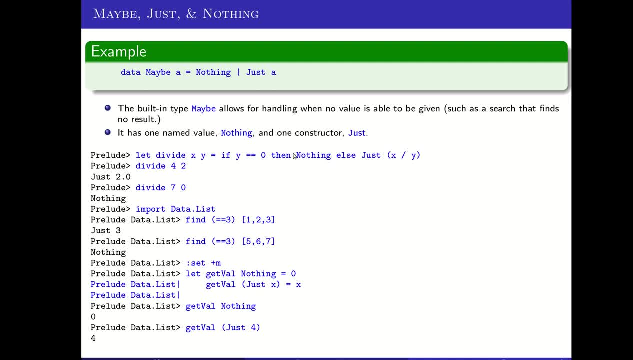 let it try to divide by zero. I want to give nothing. Now, the trick to this is that that means I'm not returning just, I'm not returning a number, I'm returning just, and then the number which I can't do- divide with- For instance divide- takes two regular numbers, So I'll have to pull. 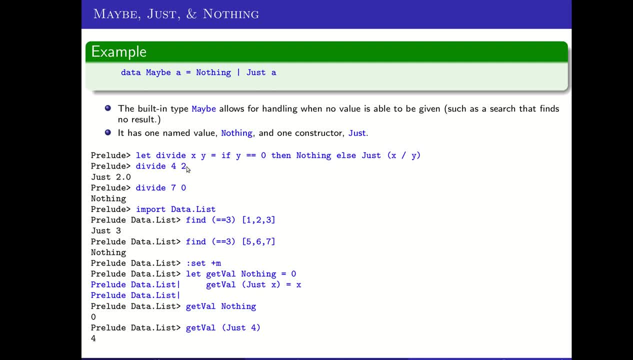 out the 2.0 from that If I want to actually do more math with it. this can make things a little complicated, And that's why this is not as straightforward as how, in many languages, you can return null, and it's sort of. 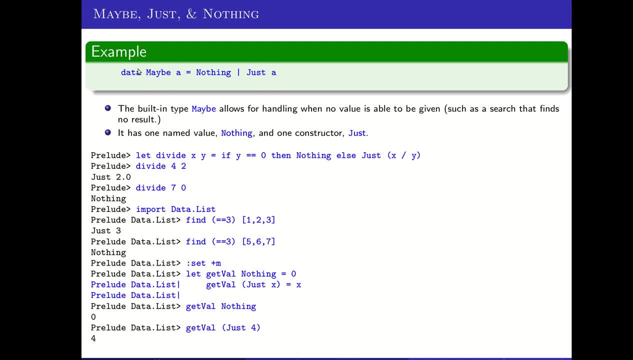 treated like any type. Well, here it actually has to specifically be the maybe type. So the find function in datalist can take some criteria and see if there's anything in the list that matches the criteria and return you the first thing in the list that matches it. So if I look for something, 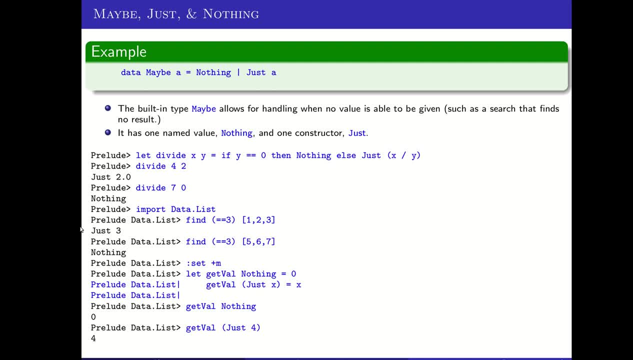 that's equal to three in the list one, two, three, it will return me just three. If I look for something that's equal to three in the list five, six, seven, it will return me nothing. Here is I've defined, I've set the multi-line so that I can show you a multi-line function in this example. 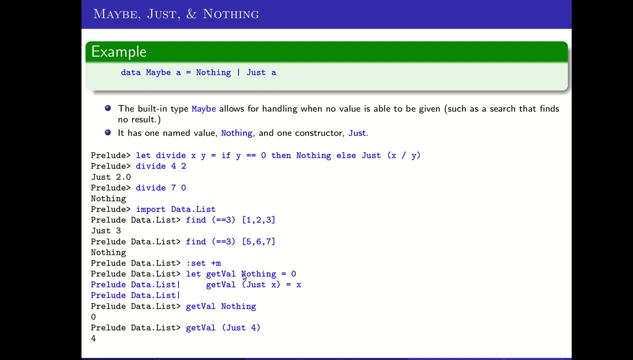 And I want to remind you that that's there so that you can use it when it's necessary for you. Um, so then I've defined getVal if there's a nothing to give me zero, for instance, And I've defined getVal when it's just a value, to give me out the value from it. Now you want to be careful. 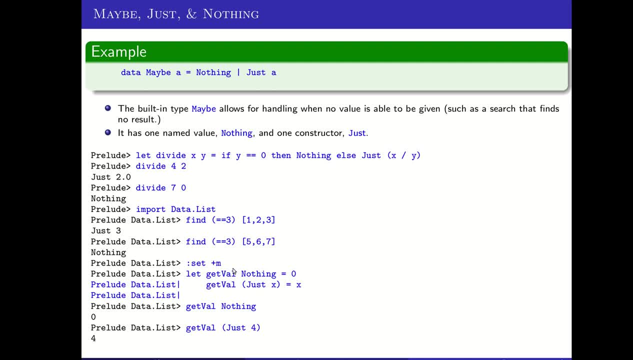 in using something like this, because what you provide as your nothing could cause problems if it could have been one of your real values. So you want to be very, very careful in trying to pull out the something from the just if your nothing value really can't. 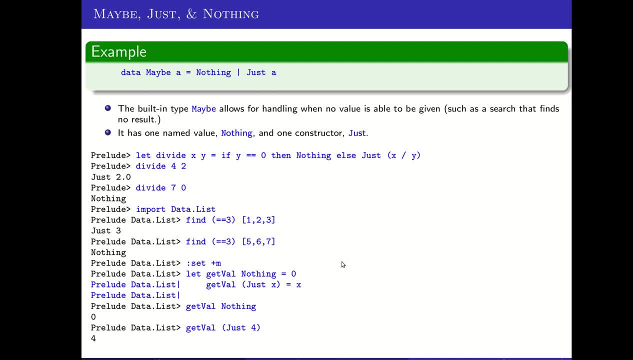 make sense, And so these maybe types can be pretty complicated for beginning Haskell programmers to work with because of that fact that you can't just say, um, find the thing in the list and then add it to twelve, for instance, because you can't add twelve to a maybe, You can add twelve. 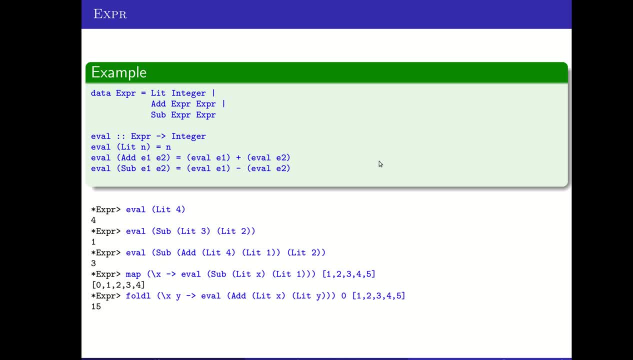 twelve to a number. Here's another type that we're defining that will allow us to define expressions, And this is a pretty simple set of expressions, but we could define a more complicated set of possibilities for expressions. We've got literals that are integers in my 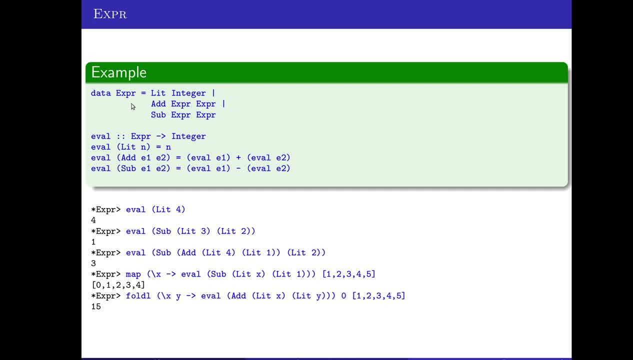 expression setup here, And then I've defined addition and subtraction for them. So a literal is a constructed type that takes an integer And add is a constructed type that takes two expressions, And a sub subtract is a constructed type that also takes two expressions. 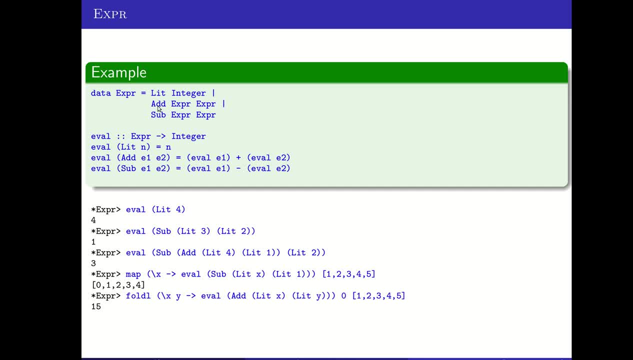 So you'll notice that the type is used inside of itself here, that we're able to say we can make expressions of expressions. That allows us to do things where we could add, for instance, the results of two different expressions, And we'll do that down below. 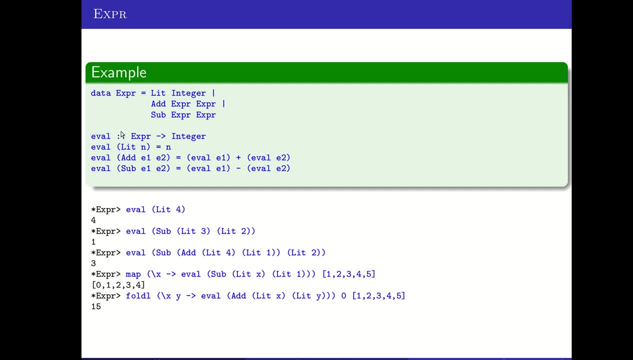 So here is a function that allows us to evaluate expressions. It takes an expression and gives us an integer as a result. Eval on a literal will just give us the value, the integer value, from that literal. Eval on an add will take the two expressions that the add. 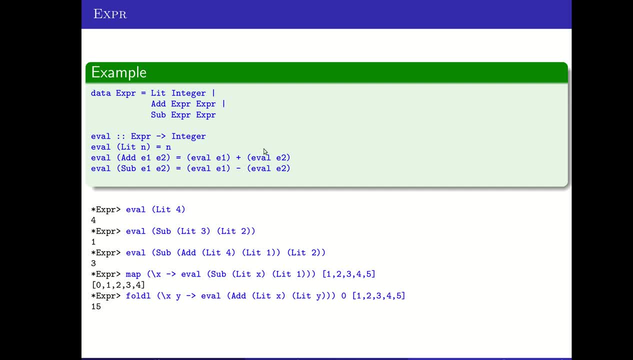 has as parameters and call eval on each of them. Summing their result, You can imagine that this might lead to more eval calls, and more eval calls and more eval calls, if each of those expressions was complex as well And sub does the same thing. Taking the two expressions, 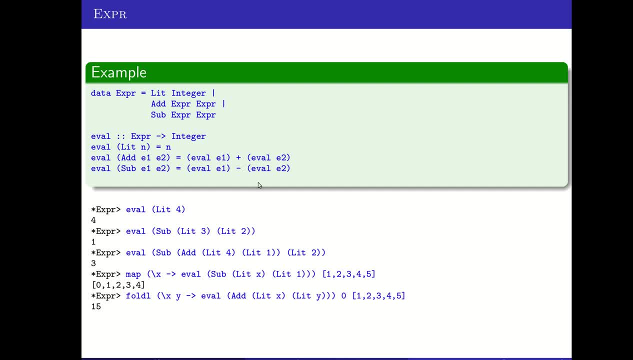 evaluating each of those expressions and doing subtraction on the result. So here's some examples: Calling eval on the literal for gives us for out. Calling eval on sub 3 and the literal 2 gives us a result of 1.. Eval on sub where one side of it is an add expression. 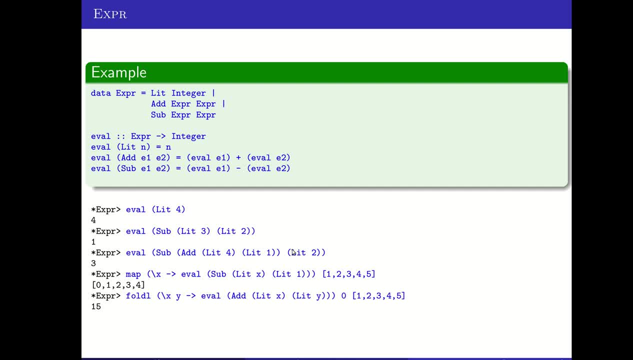 and the other side of it is just the literal 2 as an expression. So here we are adding 4 and 1. that will get evaluated to 5 and then we'll get to add it or, I'm sorry, subtract the away, the 2. 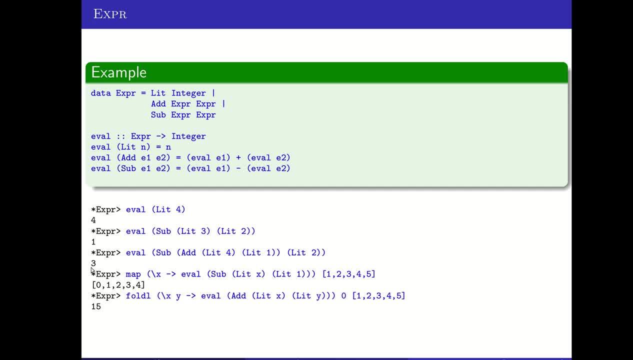 in that literal over there and get the result 3.. Here I'm mapping the anonymous function that takes an x from my list and does sub of a literal with that x and a literal: that's 1.. Now this is a pretty complicated way to do subtraction. just minus 1 on each item from the 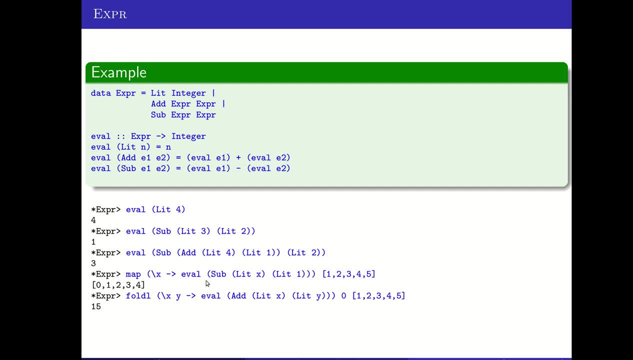 list, but you can see that it provides us a tool for building these sorts of expressions, and so we can build complex things even using pretty simple and small types like this, where we could define our own sort of little sub language in Haskell- and Haskell has been used to construct scripting languages and other sort of linguistic. 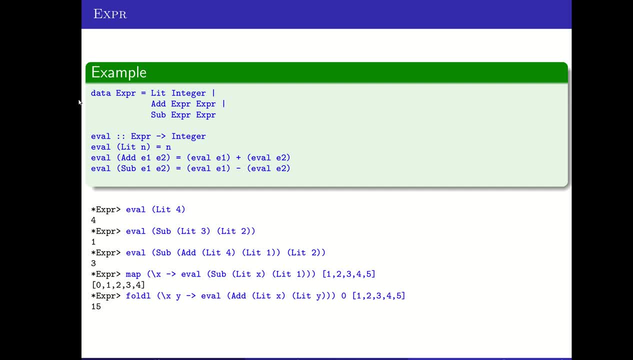 things, and so this kind of structure is not that unrealistic in Haskell in real applications. Here I'm folding where I eval, adding x and y, and those x and y are just summing my list that I was given here, so this is equivalent to folding plus over that list. but again I'm using this new type. 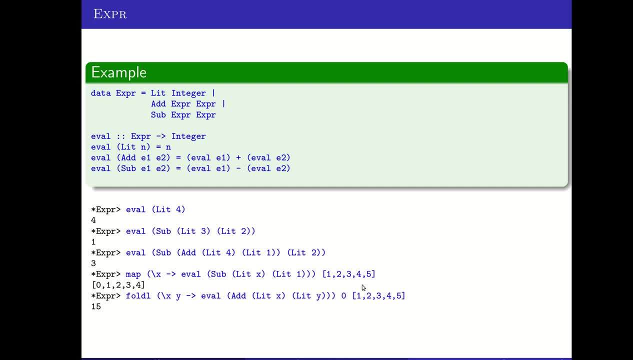 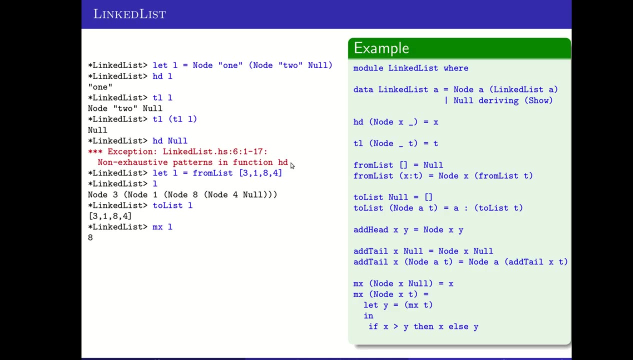 that I've built that uses expressions in this constructed format here. So that's kind of neat to be able to build sort of our own language inside the language by building what expressions can look like. We also can define full fledged data structures using these data types in Haskell. So here: 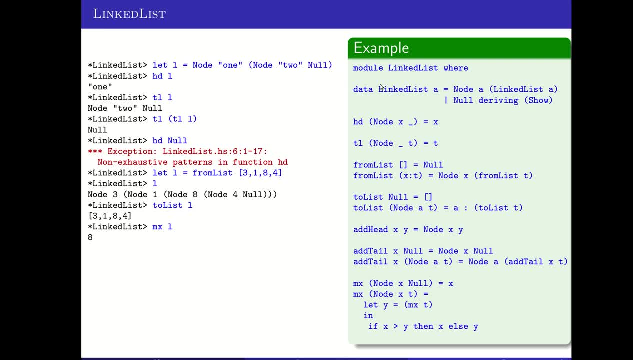 I've defined a module for linked list where the linked list types take some input, type A. This is like a generic parameter in Java or a template in C++, so it takes that A And so a linked list of, As will look like This: 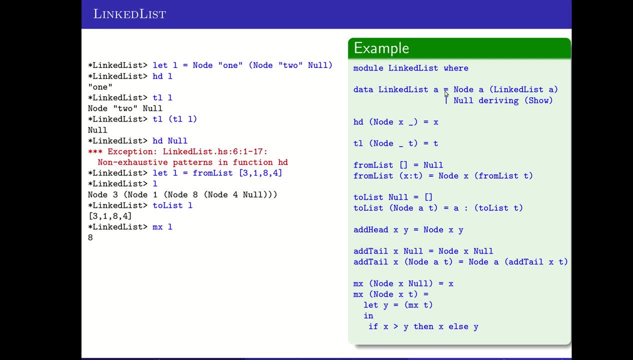 Either it will be null, which is the empty list, or it will be a node of A that points to a linked list of A. So you can look at this parenthetical part here as being like the next pointer in a C++ or a Java style linked list. So the next. 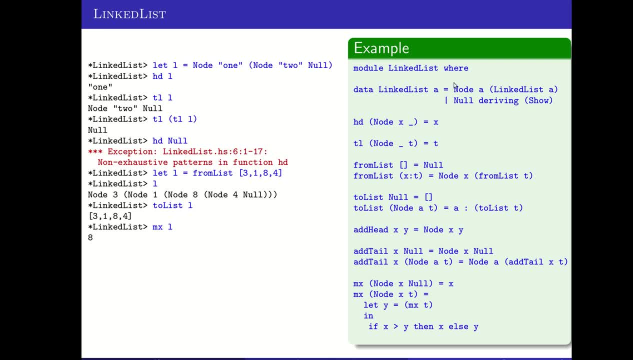 pointer is just defined by saying that a node can have a linked list as its next and in fact must have a linked list as its next. Now that linked list that it has as its next may be null and eventually should be null for our lists. 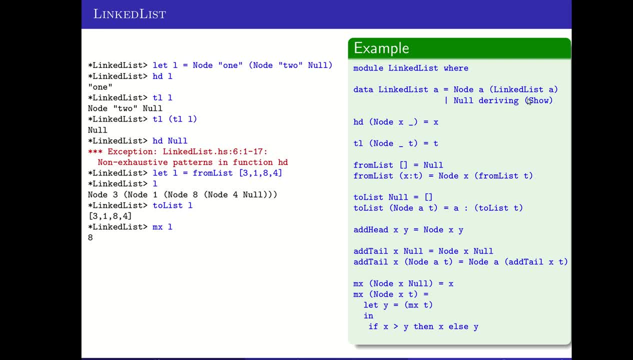 to be constructed. I've derived from show so you'll be able to see the linked lists. but you'll see that it's in this sort of default format. So the head of a linked list, well, head, if there's a node, we get its X and we return that X Tail. 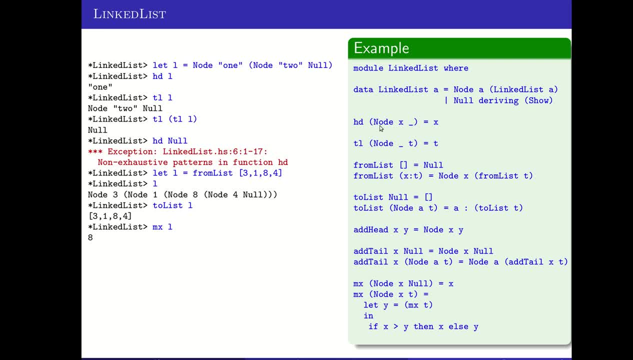 if there's a node, we ignore its value and we take that parenthetical linked list part, which we've called T here because it is the tail, and we just return that T. So here we can see some examples here. L is defined here as node, with one as its. 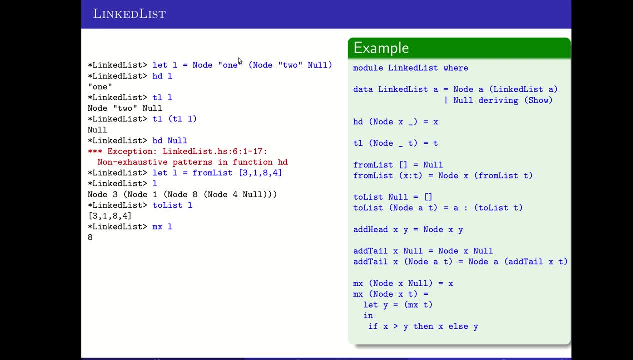 value. and then it has a next, which is a node with two as its value, and that node's next is just null. So this is essentially a two node linked list that ends with that null there. If I ask for the head of it, I get one. 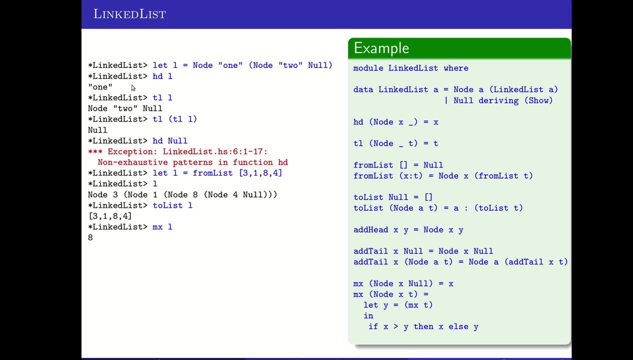 because that's the value of the first node in the linked list. If I ask for the tail, I get the node that has two as its value and null as its linked list. next Here, if I ask for the tail of the tail of L, 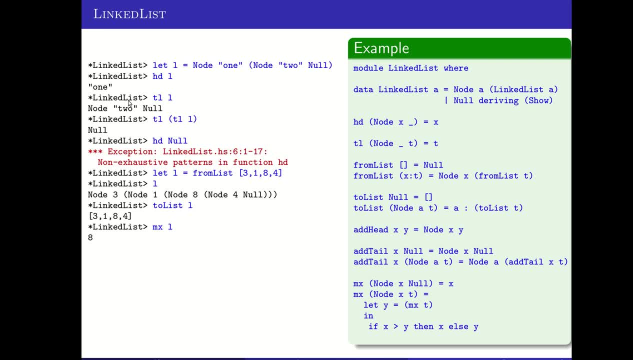 well, the tail of null. that is null If I ask for the head or the a tail of null. in the way I've constructed these I left a non-exhaustive pattern in there, So it will cause some errors if you ask for the head of null. but this isn't that unreasonable, because 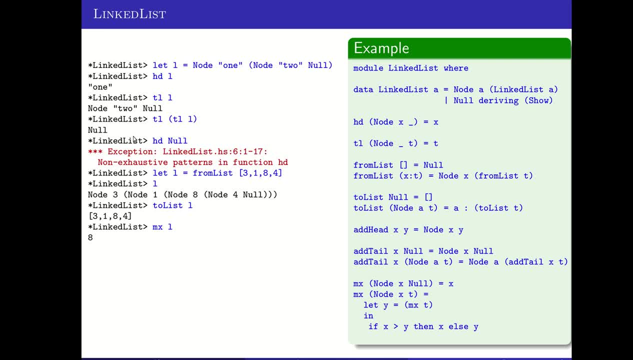 the same is often true in the case of asking for the head from an empty linked list. in other languages too, What kind of error you want to indicate and how you want to do it could vary. We could, for instance, have defined one where it said: head of null is equal to nothing, and this is 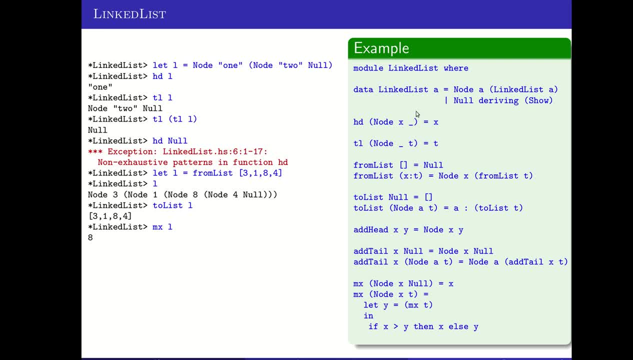 equal to just x, and we could have used the maybe type for it. but as we saw before, those can get complicated, So here I've just allowed it to cause an error- maybe not the most helpful error in this case, and there there's definitely room to improve on this module. So, however, I've also given some 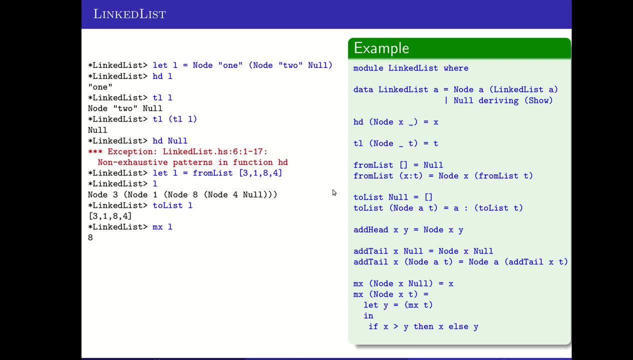 nice ways to construct and to get the values from the linked list. So we can go from a list to a linked list recursively here. If we have a list that's empty, well our linked list is null, and if we have a list that has some, 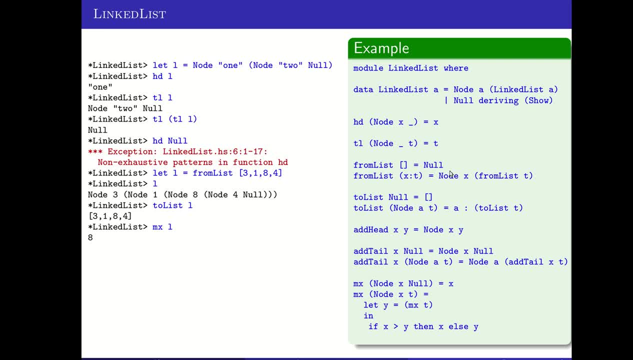 head and some tail. well, we make a node of x, and then its next will be the result of from list on the tail, And so this will keep calling recursively until it hits a null or an empty list as the tail, which will give us null as the tail. 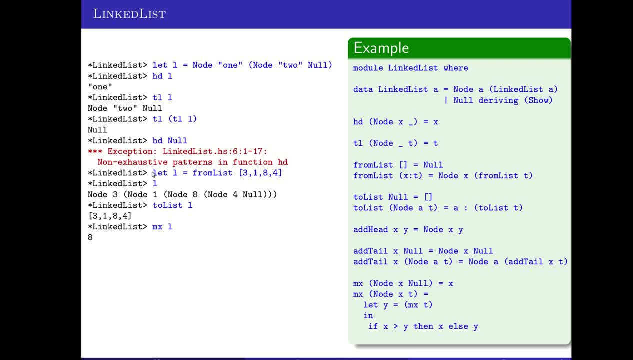 And that's the last next in our list, And we see that here. Let l equal from list 3, 1,, 8,, 4.. Well, it constructs a node with 3, and then for its next it constructs a node with 1, and for its next, 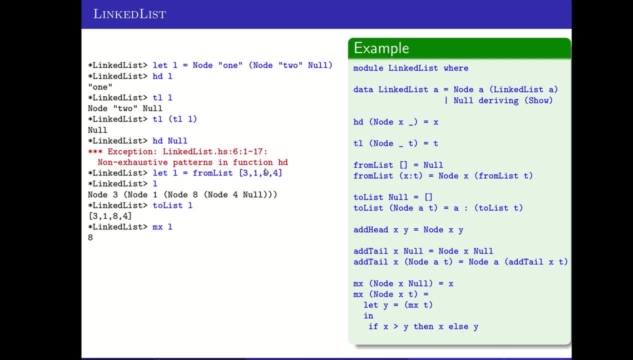 it constructs a node with 8 and a node with 4, and then, finally, the tail would have been the empty list. and so it's next, after the 4 is null. If I ask to go to list, well, that will walk through until it's a null. 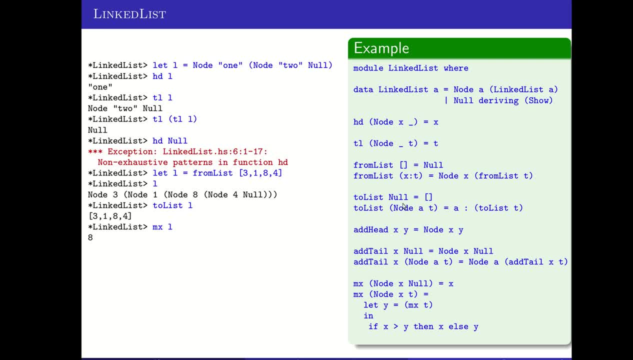 when it's a null, it gives an empty list, but when it's not null, it gives the value a, combined with the result of calling to list on the tail. and so, again, we're recursively defining this data structure, as you can see in the way that it's shown here, and we're recursively being able to build and pull apart the. 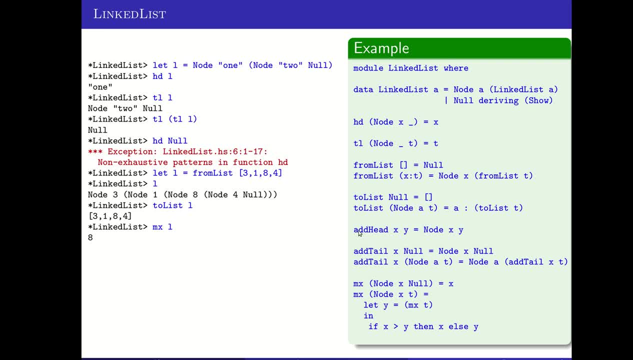 pieces from it. an ad at the head is actually really easy. if we want to add head of X to some existing linked list Y, then we create a node X Y. I probably could have named this L or something to make it a little clearer here this part. 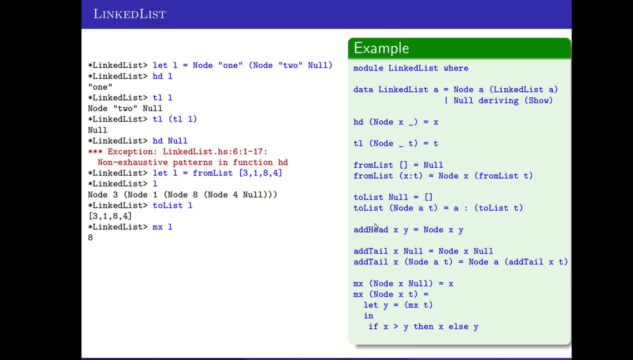 is an existing linked list. I want to add X as the head, and so I just return a node that has X as its value and the existing list as its next. now, bear in mind keeping that functional mindset. this does not change the existing list. you can use a node here by hand to create a new list. this returns me a new list and 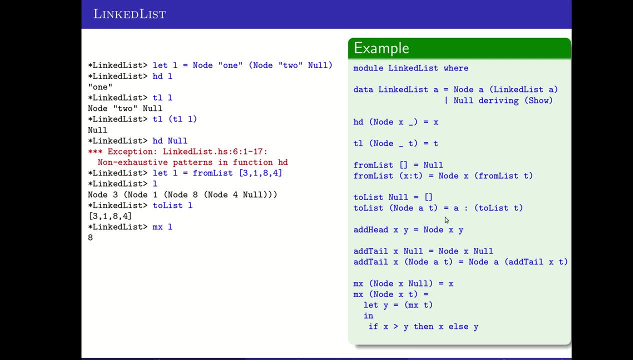 so we have to be careful that if we're trying to add head, we're actually doing something with the result of that, not assuming that that changed. the list that exists here- add- tail- is a little more complex, because if you're adding at the tail, you have to actually get to the tail. if it's a null list, well, that's easy. 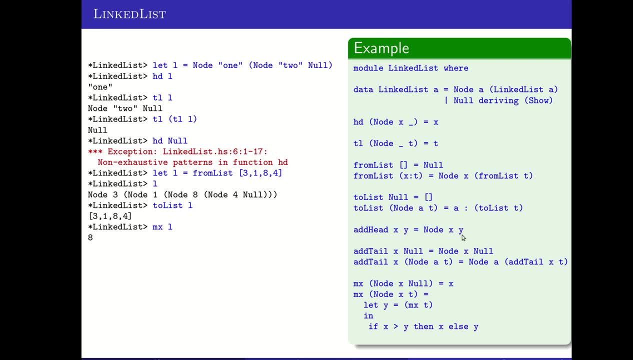 because I can construct a node with X as its value and now we have a list. So what I do up to there is I recursively call with x and node and a node that has some a and then some t tail, I reconstruct the node to have node with a as its value and its. 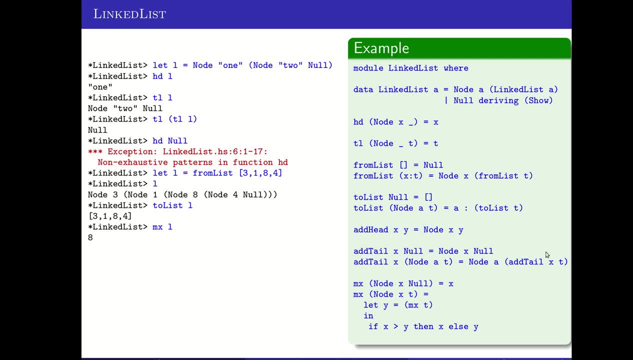 tail will now be whatever the result is of add tail with x and the existing tail. So what this will do for most nodes is nothing at all. It'll just reconstruct that node and it will eventually get the next that it had. But for the node that had null as its next, then it will get a new node. 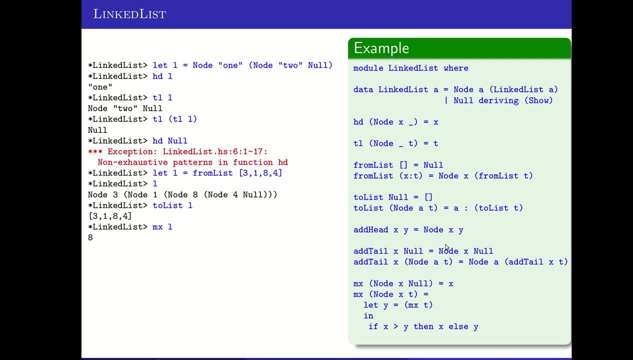 as its next. that is the node with x as its value and null as that one's next. So it extends my list by one more And again, bear in mind, it does not change this original list. It returns me a whole new value that we have added. So I'm going to do that by changing this value to null as 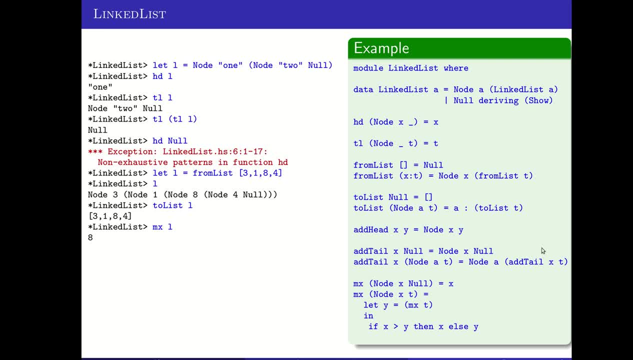 that one's next. So that's what I'm going to do. I'm going to continue this dataõm by changing this dataõm. just bearing mind it does not change this original list. It returns me a whole new, whole new list that has that one value added. Now there are intelligent ways that these are. 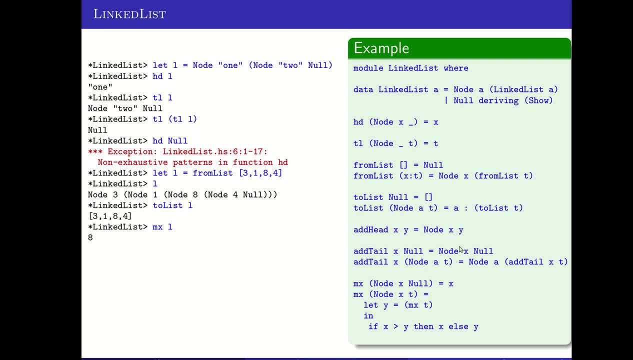 handled in the background in Haskell, so that you are hopefully not always creating huge whole new lists but are reusing some existing stuff that's stored in memory. but don't think of it as changing the original list, because it will not. It will give you a new version of the list that has that. 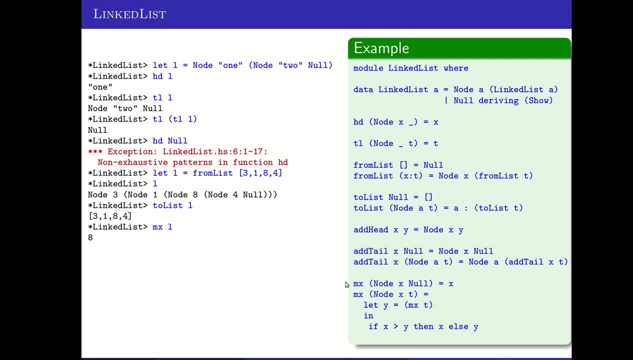 extra value added on. And here just to show how we would sort of step through the list and find something is a max function for this type of list. If you have a node that's only x and null, it gives you x because the singleton list always has x as its max. Otherwise, if it has x and some, 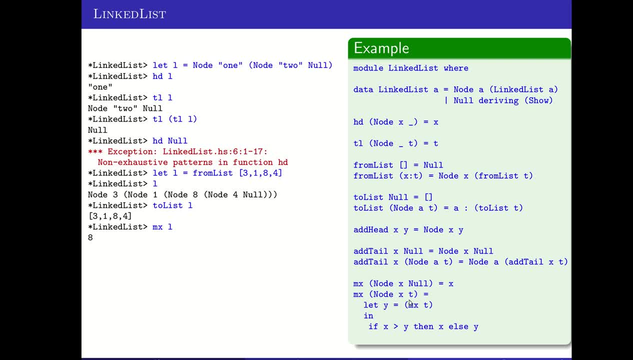 tail. well, it's going to look for the max of that tail and it's going to either return you x. or it's going to return you x If x was larger than that max of the tail, or it's going to return you y if x was not larger. 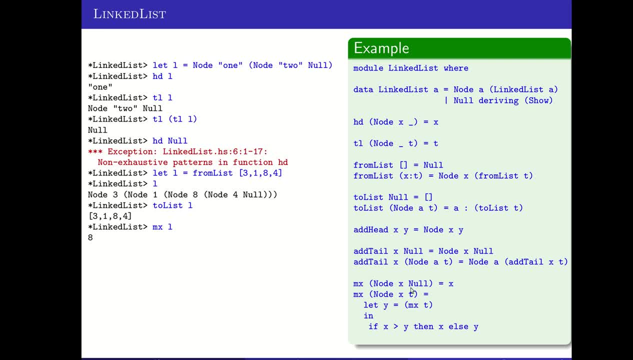 than the max of that tail. So it's recursively calling this max function until it reaches the tail, gets a max for the tail and then is able to compare coming backwards- Not tail recursive, but will nicely find the max for any non-empty list. For an empty list it would error, just like. 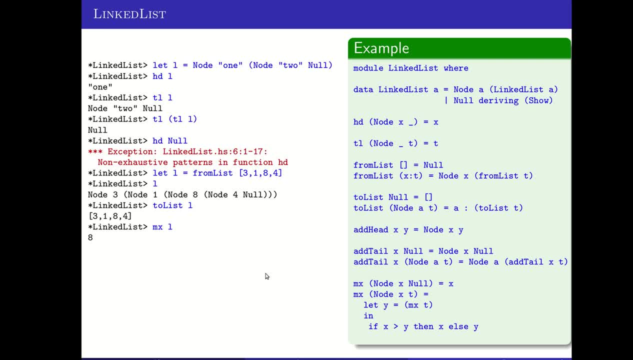 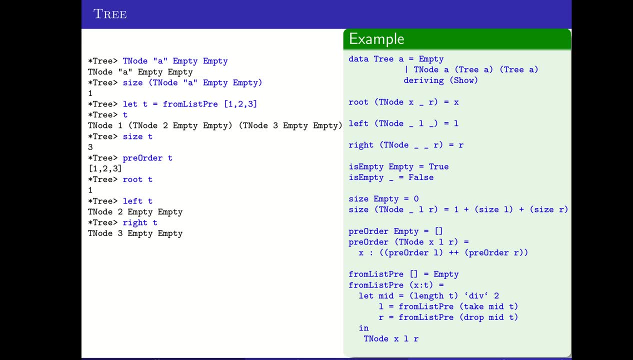 my one above. You can decide how you would want to handle that in practice, All right. and if you thought that that wasn't a big enough type of data structure to be able to define in a functional language, well, let's try trees. We can even define trees in Haskell. 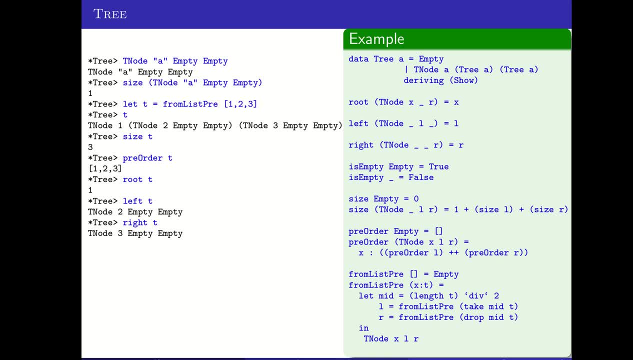 using these new data types. as we define them, We can define a tree of a's to either be empty- and that's a sort of a tree of a's- or a tree of a's to either be empty, or a tree of a's to either be empty. 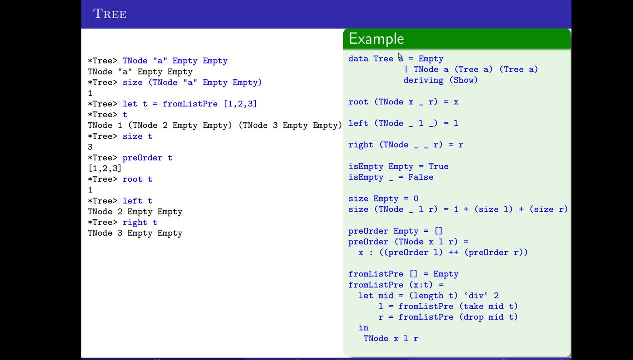 And that's a sort of a tree of a's. It's a special type that's named here, so we would want to be careful that empty wasn't a name that was already taken or we might want to use some longer name like empty tree some people will use, or stuff. 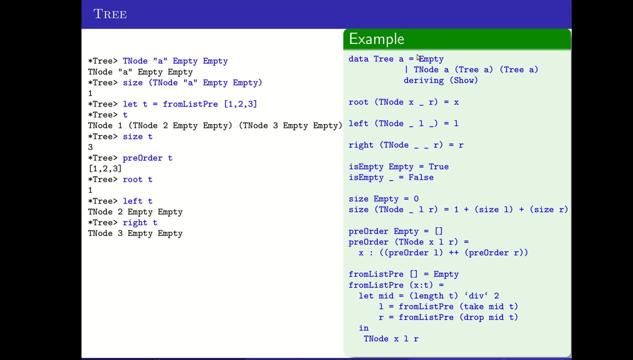 like that, but empty, is going to be one of the named types for our tree. so that's an empty tree or it will have a tree node with a as its value and a tree of a's and another tree of a's. These will be the names of the trees that we're going to use. So we're going to use a tree of a's and another tree of a's. 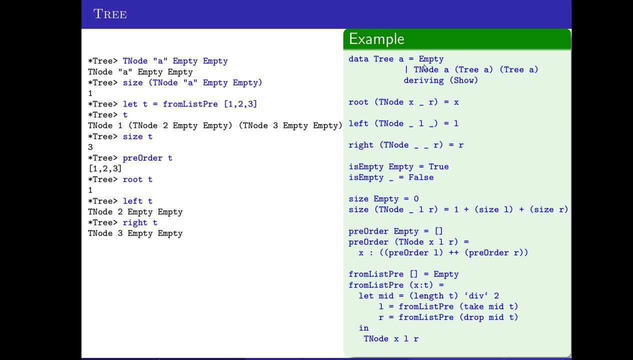 functionally the left and the right. Remember that a is not an actual variable name. a is a type name here. so we have a node of a and a tree node of- I'm sorry, and a tree of a's and a tree of a's. 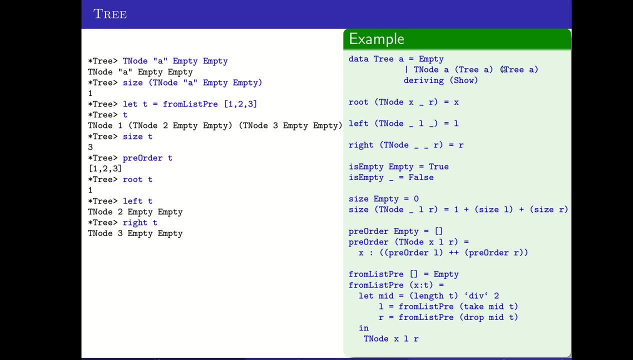 These are sub trees- left sub tree, right sub tree- and it gets a little nasty when we have to write them out. So, for instance, if I take just the tree that has a single item in it, we have to define a tree node with that single value. 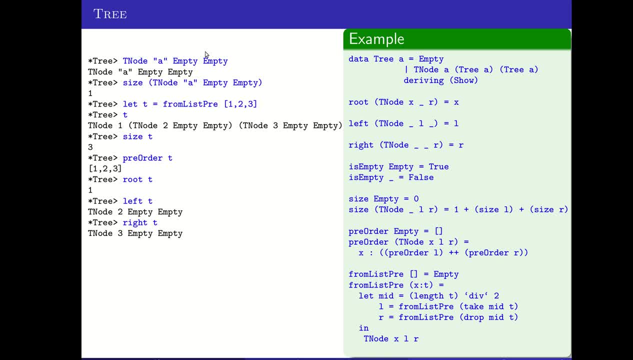 or that single value, and then it has two other tree or other trees that are empty and empty. Those are its left and its right, and so we might eventually want to write some nicer ways to display this tree, but for now we see that's a node that has a value and no left and no right. 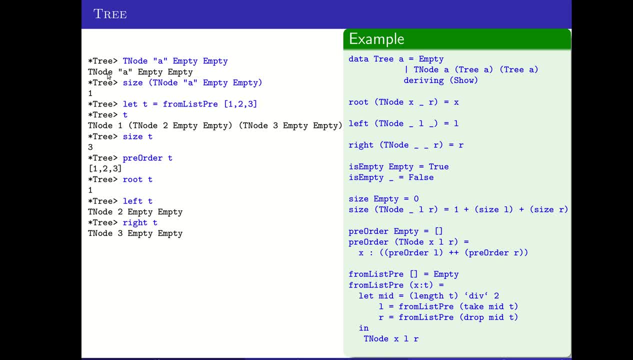 So it's a single value tree. We can ask the size of that tree. I've defined a size. if it's empty it's zero. otherwise we do one plus the size of the left and the size of the right, where l and r are those second trees or, I'm sorry, the 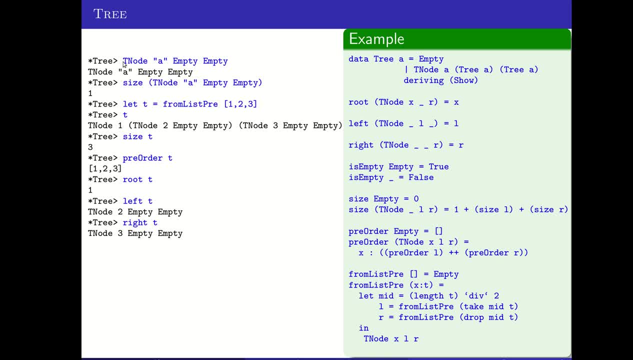 first and second trees that are defined inside of the node. So in the case of this one, it would have accumulated the one and then it would call the size on one of the empties and size on the other empty, getting zero and zero, and so its result for size of the left and the right. 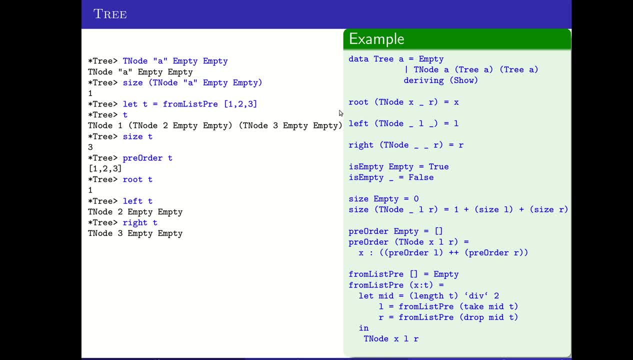 As would be one Ok and root just gives us the value of the current node and left gives us the left sub tree and right gives us the right subtree or the first subtree and the second subtree. here We can test or we can do things like put it to a list in pre-order or get it from a list as pre-order. 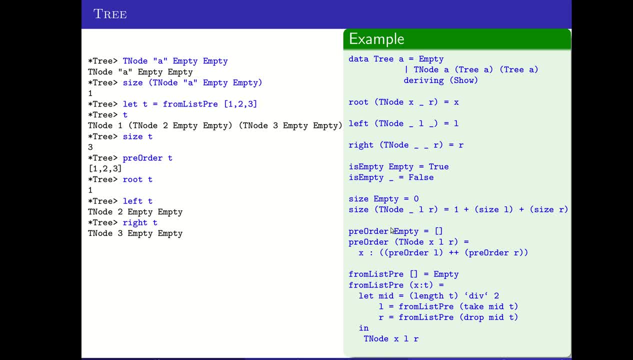 order and so to do these. it's not too dissimilar from what we did for the length list. we will, for an empty list, give an empty tree, otherwise we will. i'm sorry for an empty tree. we will give an empty list for giving a pre-order list version of this. otherwise, if we have a tree node we'll use its. 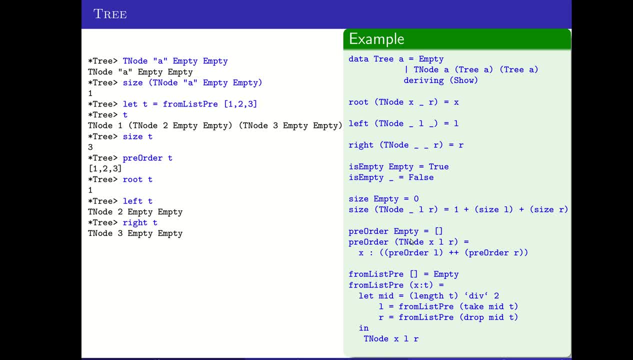 value x, remember pre-order. is this node, then the left sub tree, then the right sub tree. well, that's easy. we have x combined with the result of calling pre-order on the left sub tree, merged with the result of calling pre-order on the right sub tree, and so for my singleton tree here. 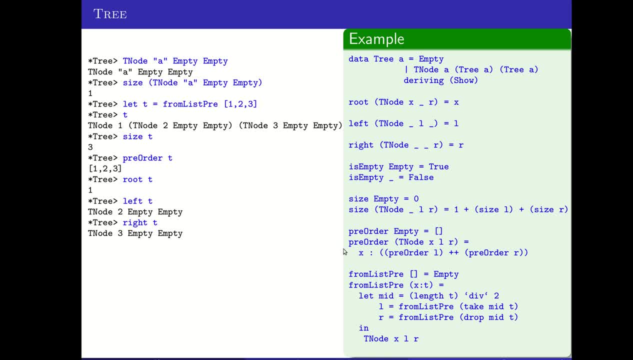 that would get called once. it would construct x and then it would end up combining x with the empty list, merged with the empty list. So it would be x combined with the empty list and we would just have that one inside of a list. I've done the opposite. 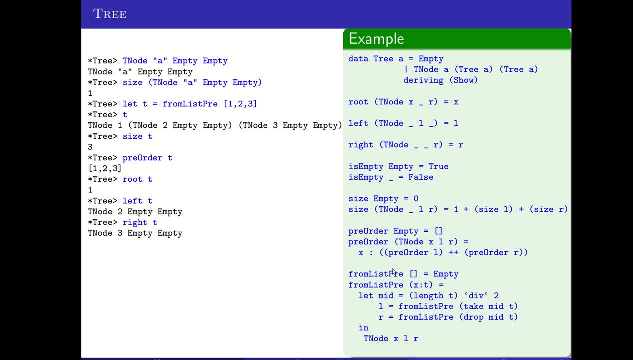 direction: getting from a list into a tree. Well, give me an empty list and I'll give you an empty tree. That's simple. If it's a list that has a head and a tail, then I will get the middle value of that so that I can pull out what should be the left subtree and the right subtree. 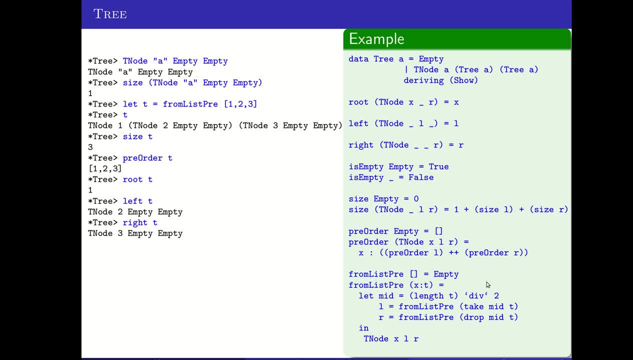 by taking the length of the tree and dividing by two, And then I get the. I take up to the middle and I drop after the middle. I'm sorry, I yes, I take up to the middle and I drop what comes before the middle, And then I'm able to create a tree node on x. 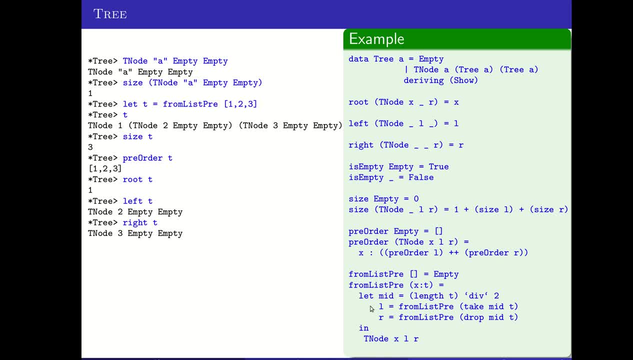 the current value and the left subtree that was created by recursively calling on part of the list and the right subtree that was created by recursively calling on the other part of the list. Um, I get the benefit also that this will be balanced, and in so far as the list is divisible by two, And so 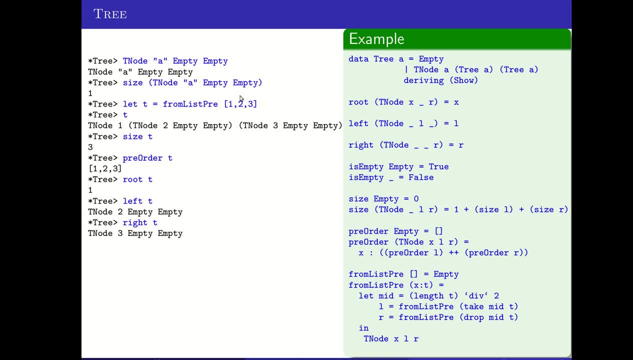 I can see that I can. I'm able to do that with the list one, two, three. It creates me a tree node with one And then the left subtree of that is a tree node with two and empty children, empty sub trees, And then the right subtree is a tree node with three. 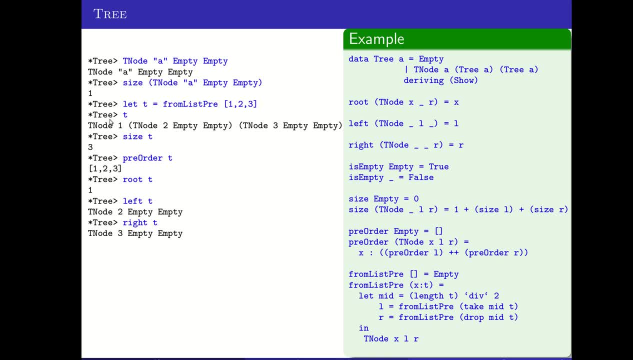 and empty left and right sub trees. The size of this will be three, because we get one for the middle And then we recursively call on the others to get one. It's if we ask to put it into a pre order list, then we will get out one, two, three again, because one was my root and two and three. 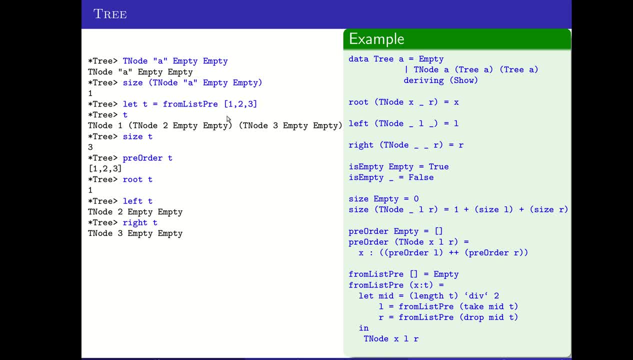 were its children. bear in mind, this is not any special kind of tree other than a binary search tree. You could, however, write code in Haskell to generate, for instance, a binary search tree or other types of data structures that you wanted to, all by being able to define, maybe some named. 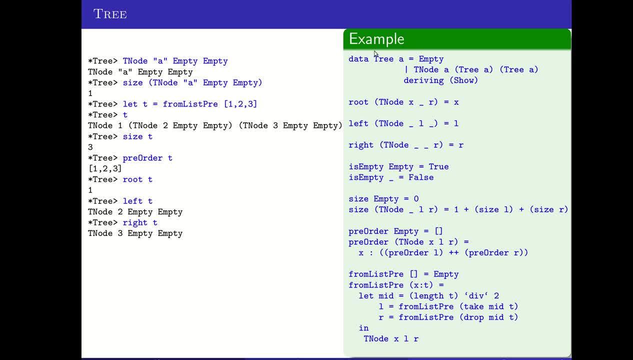 types and some constructed types, especially when those constructed types can be recursive and hold on to more and more Of the values of the types that you're wanting to store in your data type, And so you can see that constructing new types in Haskell has a pretty wide range. We can define some really simple ones. 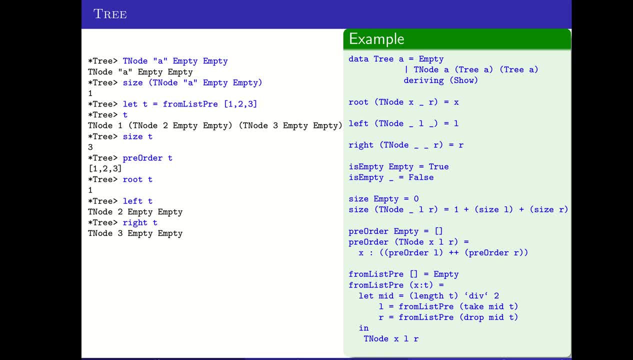 that only have a few named values. We can even define ones that are constructable with just some of the primitive values, like ins or strings, Um. and we can define these complex, recursively defined types that allow us to build full featured potentially, if you want to put the work into it. 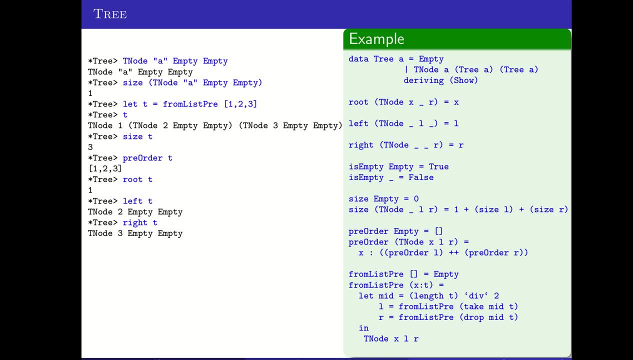 data structures within the language And they're still following that Haskell in that functional mentality and style of being recursively defined and being immutable. When I add something to them, I'm generating a new linked list or tree or whatever the data structure is, and still 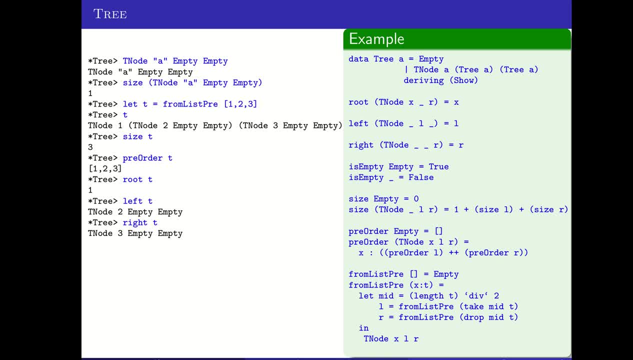 having that original kept as it was, to be able to do whatever I need to with that newly derived type and possibly still revert back to the original if I return from a recursive call, for instance, or things like that, And so you'll get some experience with doing a. 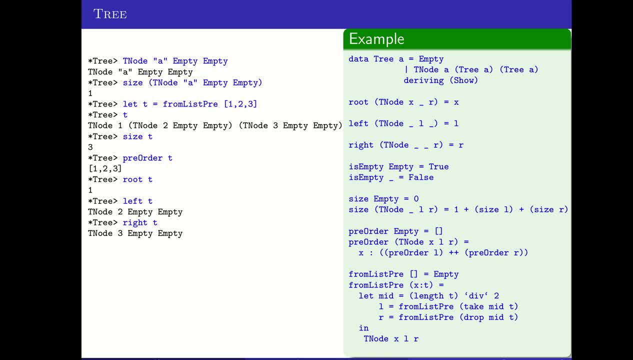 range of different possible uses of these user defined types in Haskell.